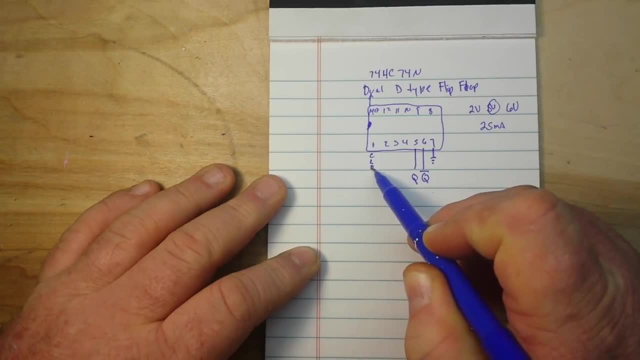 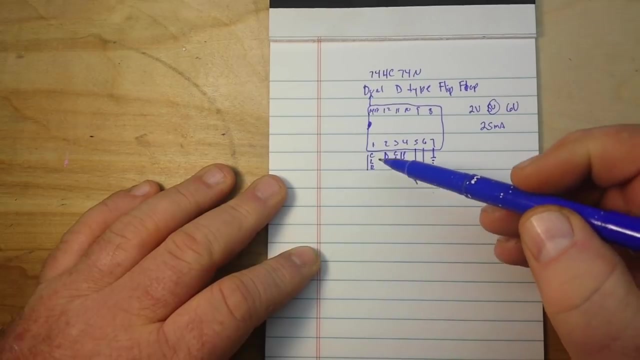 Pin 1 is our clear and it is an active low. Pin 2 is our D or data input, Pin 3 is our clock and Pin 4 is preset, also low. So for right now we're kind of going to ignore our clear and our preset. 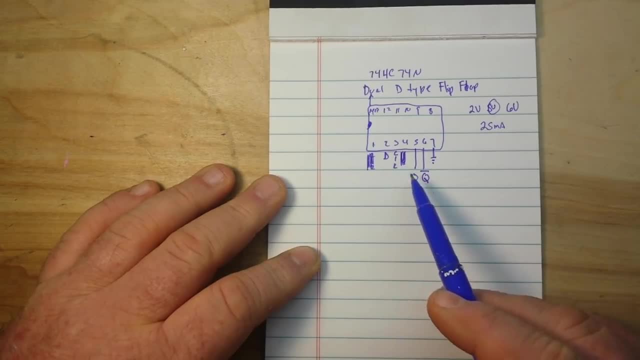 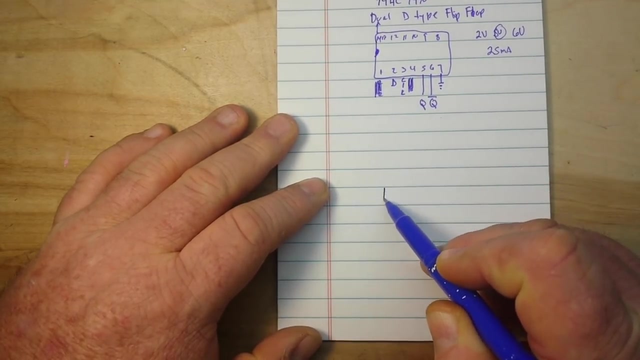 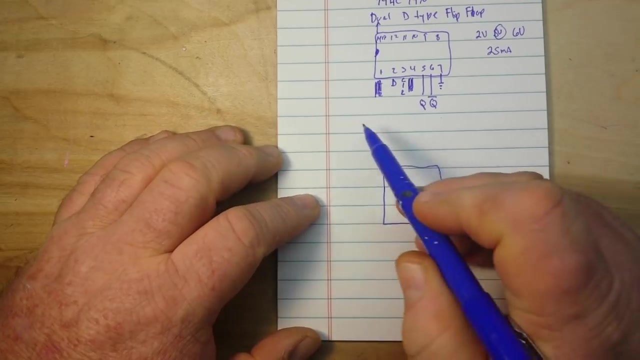 and we're just going to concentrate on our data and our clock and how they affect the outputs Q and Not Q. Okay, So let's move on to our application drawing. So we'll call this our chip here, and this will be our 5V rail. 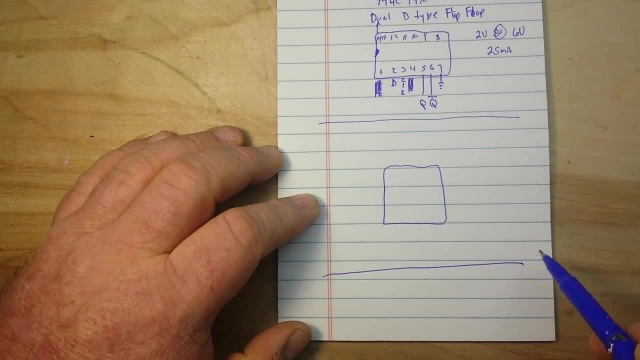 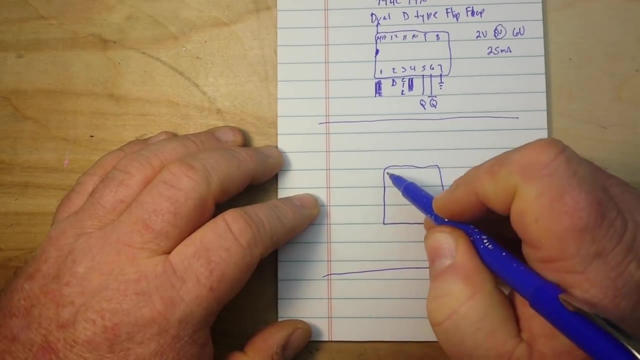 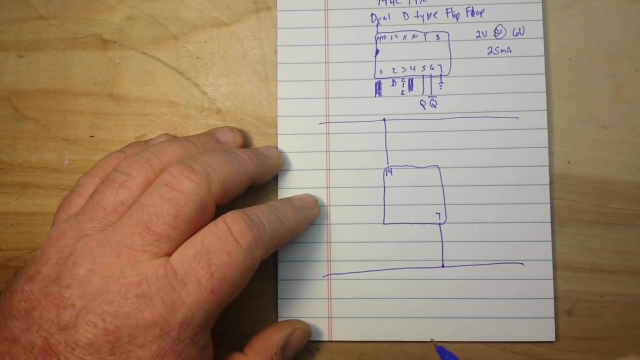 and this will be our negative rail. So again, Pin 7 to ground, Pin 14 to our VCC. Now we're going to put LEDs, because they're simple to work with, on our Q and Not Q outputs, just like that. So when Q is active, 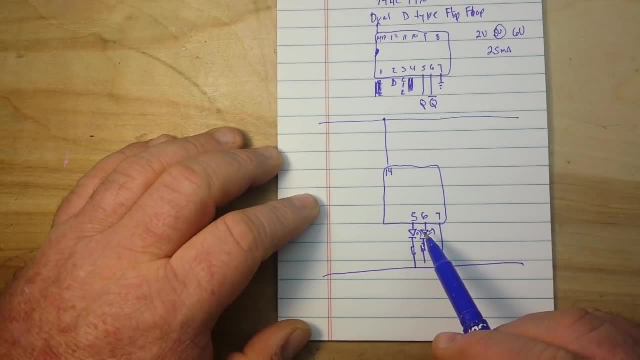 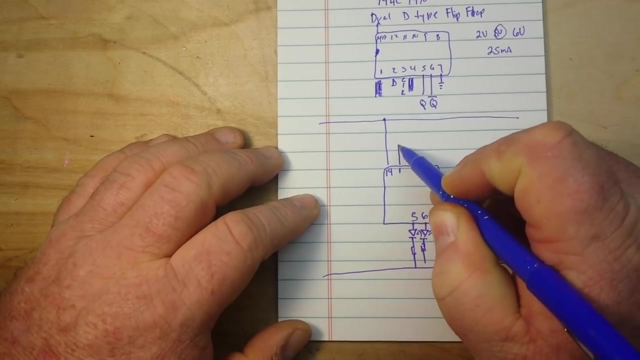 on Pin 5, this LED will light When Not Q is active. on Pin 6, this LED will light. Alright Now. Pin 1: we're going to hold high with a pull-up resistor. Pin 2: another resistor: we're going to attach an LED. 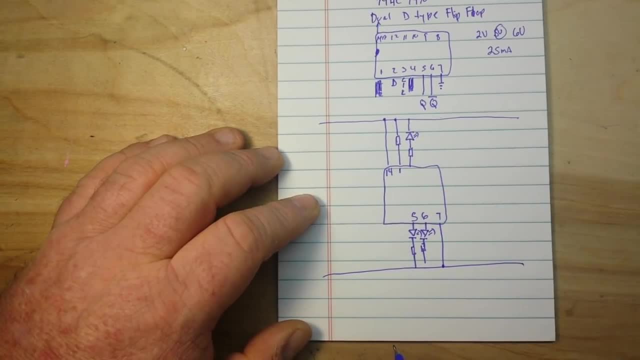 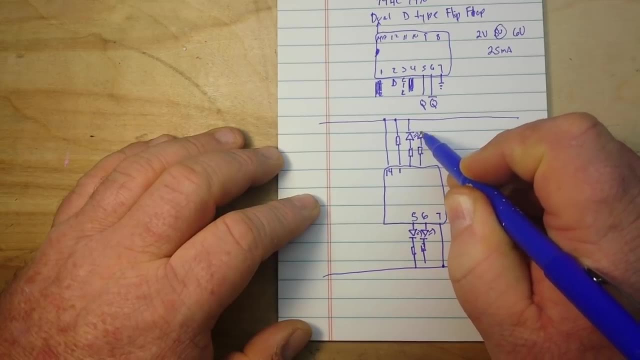 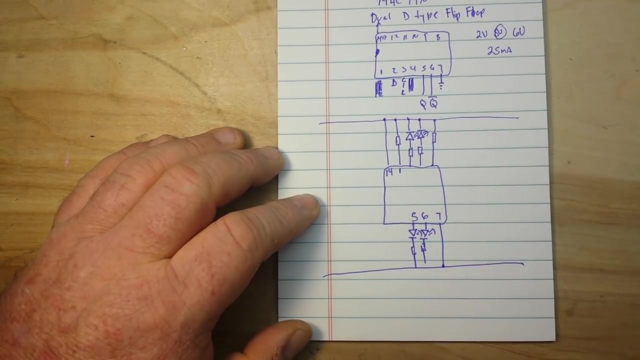 so that we can see when we're inputting data. Pin 3, same as Pin 2. pin 2, another LED so that we can see when our clock is high, and Pin 4- we are just going to hold high Now our resistor values here. 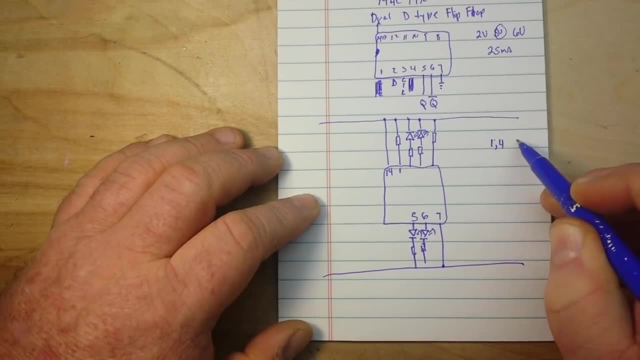 on Pin 1 and 4 are 10K standard pull-up resistors and our resistor values on pins 5, 6, on 2, 3, 5 and 6 are just a low value resistor for those LEDs, so I'm going to use 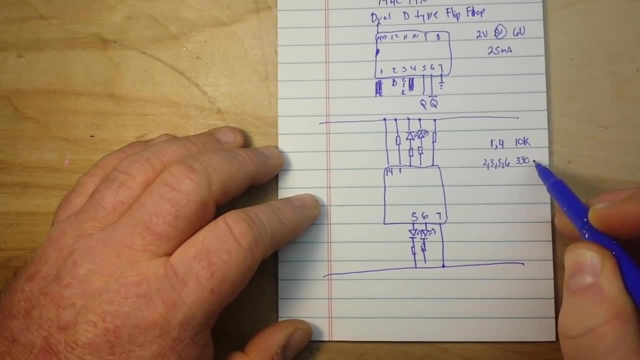 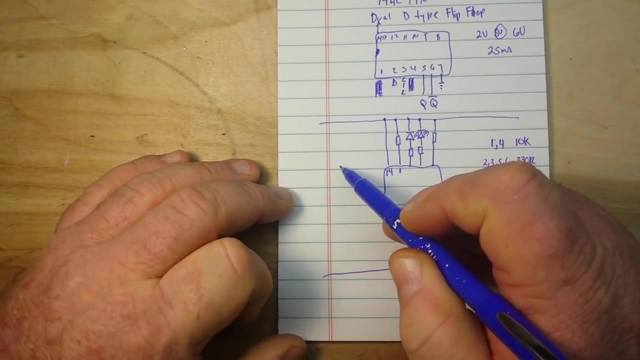 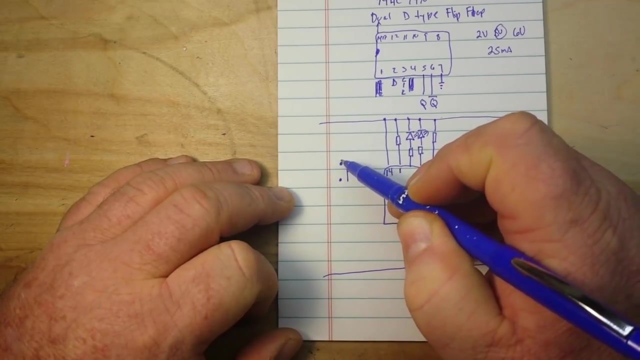 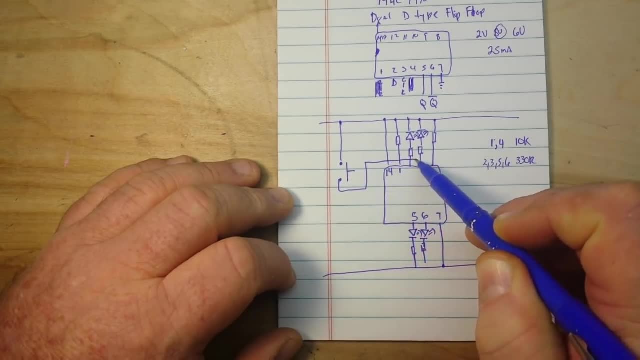 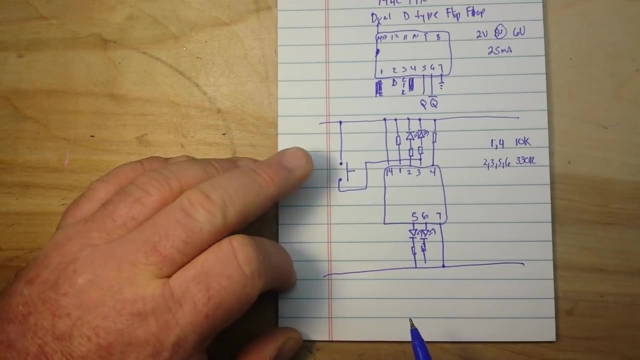 and then it is going to attach to Pin 3. I forgot to write those, didn't I? 2, 3, 4, Okay, like that, and that is going to be our clock switch, and then, on Pin 2, we're going to attach a wire. 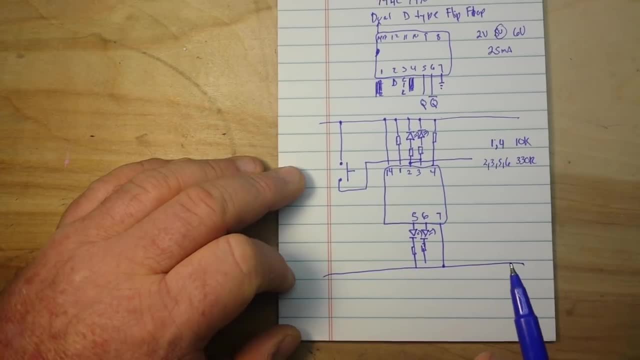 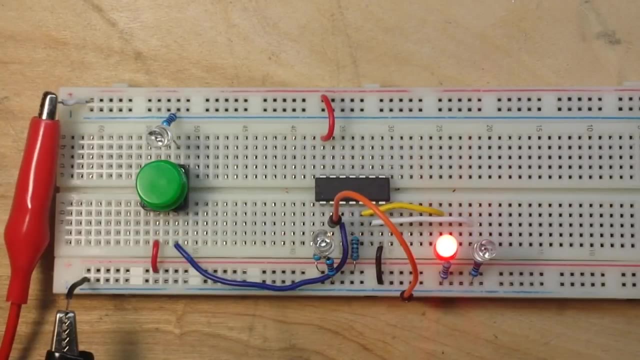 and we're going to leave it floating. The reason we're going to leave it floating is so that we can just easily move it between low and high. So let's bring in the circuit. Okay, here's our circuit, just like we talked about Our red LED here. 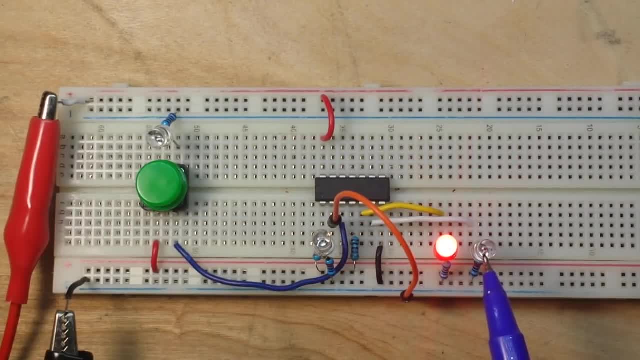 is our Q output from Pin 5. This one is a green LED and it is our, NOT Q output. Over here we have our D input. It's also a green LED, and here we have our D input. and here we have our clock input, also a green LED. 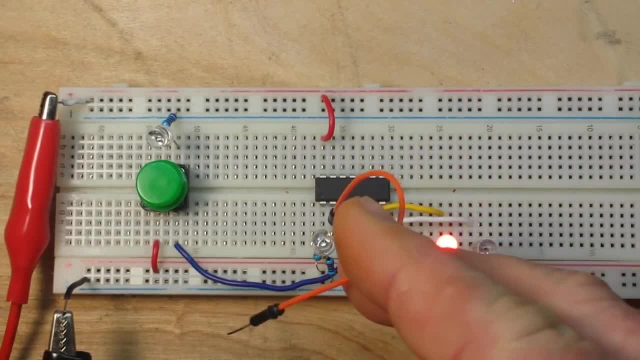 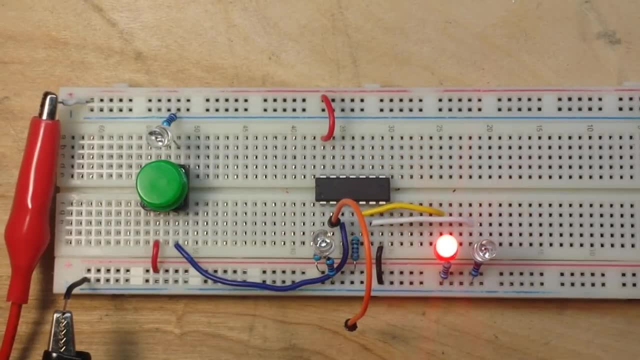 So we start out with the case of D floating and the way everything is set. our Q output is high. Now, if we bring D high- and you can see our D is now high, nothing changes. our Q is high, NOT Q is low. and if we clock it, 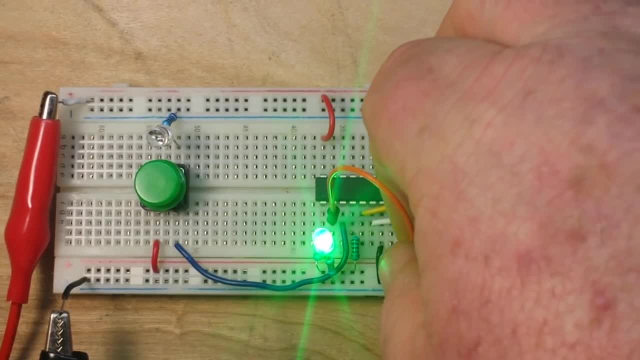 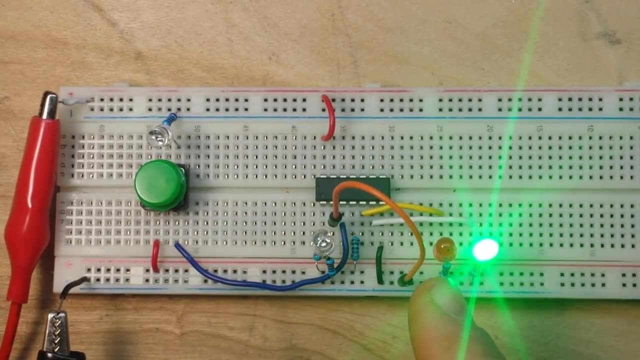 nothing changes Now if we make Q low because we had a clock pulse. I'm sorry, we didn't make Q low. we made D low because we had a clock pulse. Q went low, NOT Q went high. and now because the way the flip-flop works, 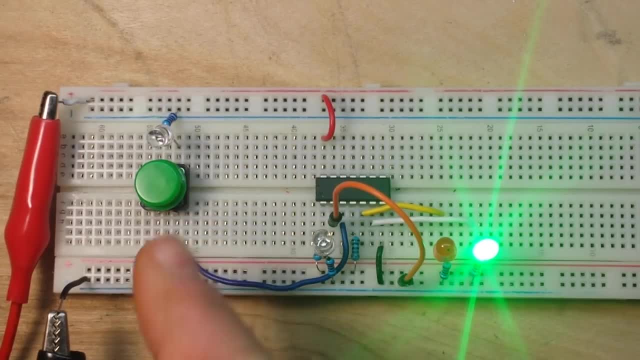 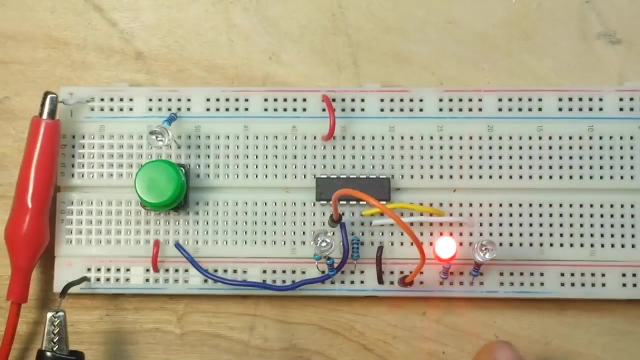 it will only change state with a clock pulse. So if I move from low to high on our D input, nothing changes until I clock it. Now we have Q high and NOT Q low, and if I go like this and bring D back to low, Q remains high. 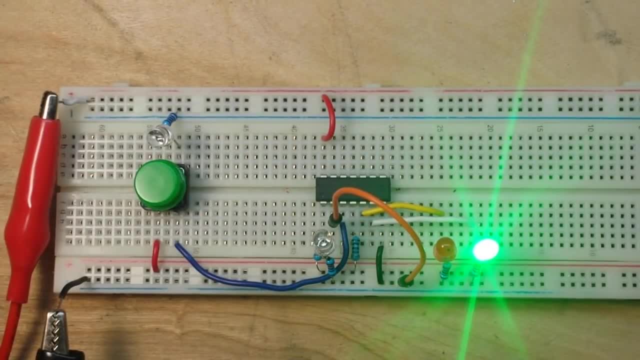 NOT Q- doesn't come high until we have another clock pulse. So basically, what we have is a latching flip-flop. You can change the state of your data input, but the output, or let's call it the memory of the flip-flop- does not change. 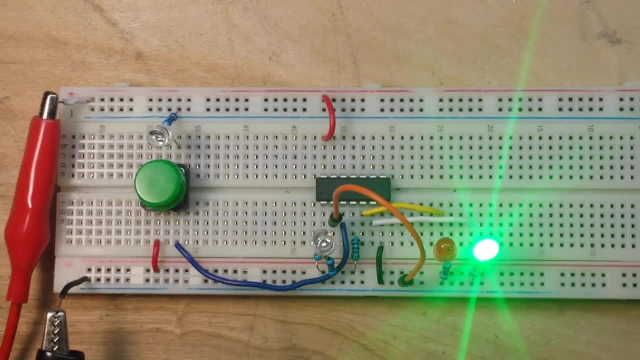 until it's been clocked. So this is basically a one-bit memory. I mean, also it's used as a high-low system for switching a couple of applications. but try and think of it as a one-bit memory. It will remember the state that you put the output in.